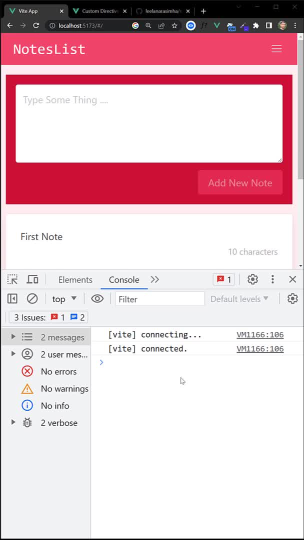 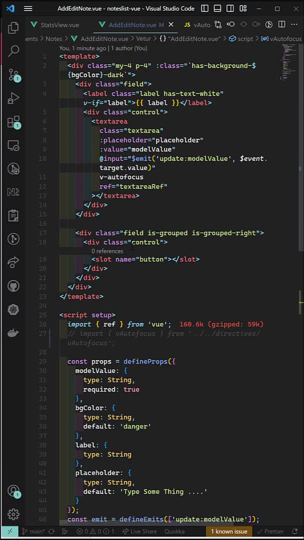 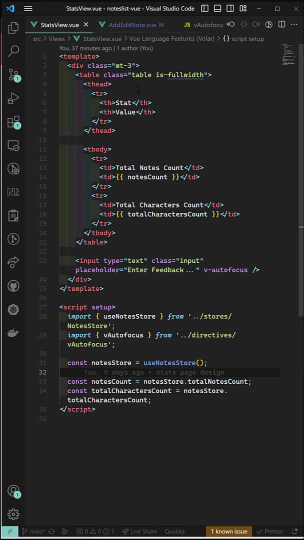 Hi guys, in this short we will see how to create a global directive in the Vuejs composition API. If you try to see here, this is our local directive which can be useful only in this component. So if you want to use this directive in another component, like stats view means, then how we can use it is: 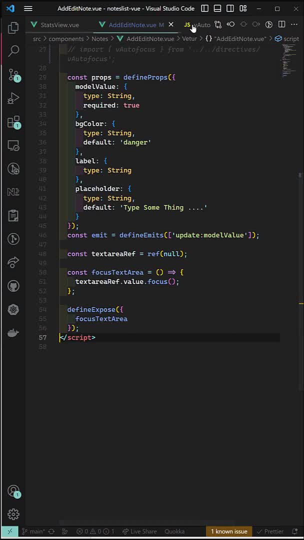 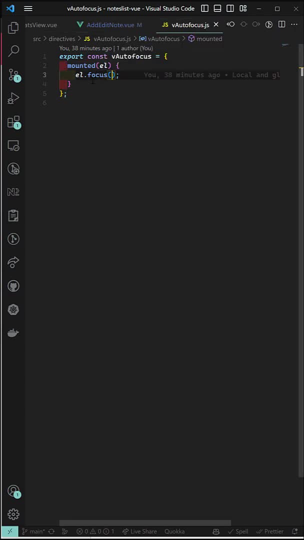 so we need to create a new file with name vautofocus. Whatever the name you want, you can create it. So this is the file we need to create and, whatever the code, we have seen it automatically. we need to paste this code and we need to use the export here. 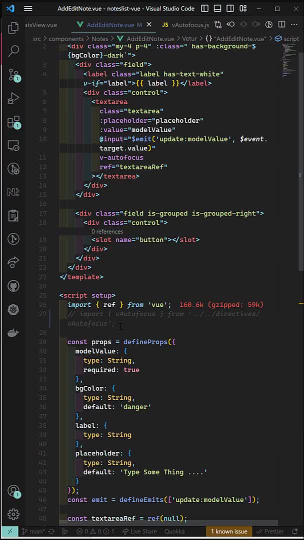 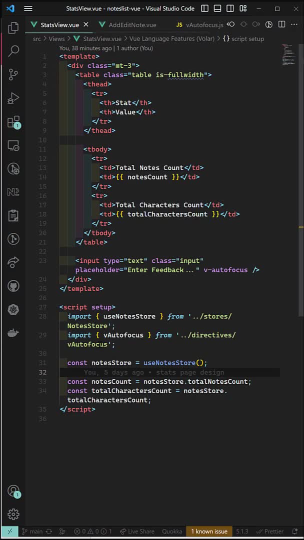 Now how we can use. it is so just: we can import this like this. So we need to import like this. So import autofocus from the directives here like this, And in the same component, in another component also, if you want to use this directive, you can use this, import like this: 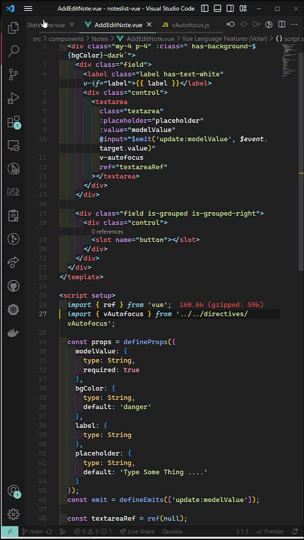 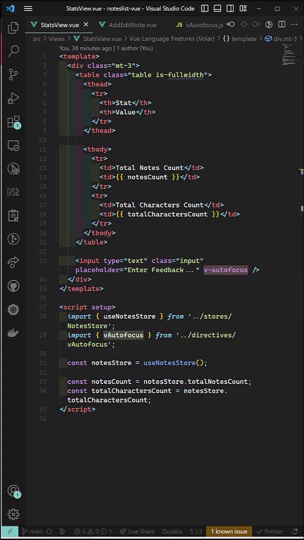 So this is where we can create a global directive and use it in all the components, wherever you need this directive, And you can use it directly, like this: v-autofocus to the input elements. 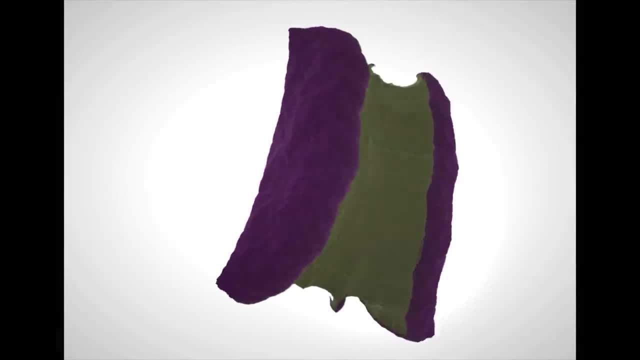 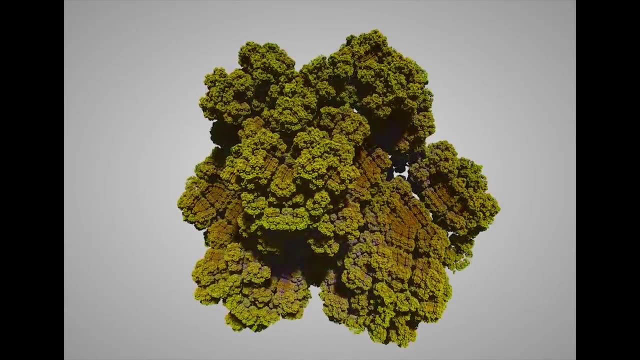 A while ago I posted a video showing some real time fractals I created, but I never got a chance to explain how it works and how you can build your own. It's actually super interesting with some really beautiful mathematics and tricks I'm going to do. 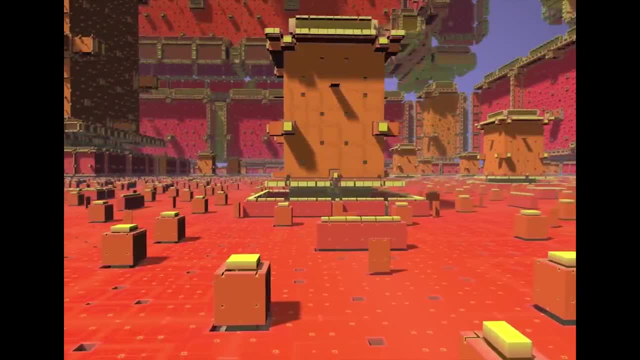 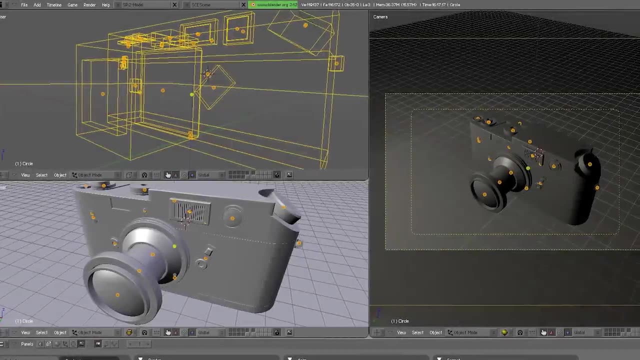 my best to explain everything and hopefully at a level that everyone can follow. I'll also be sharing the source code so you can try it out yourself. So at the very basic level, we need to first understand the different types of renderers. 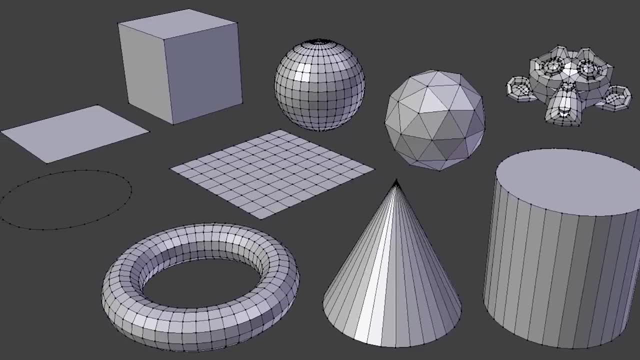 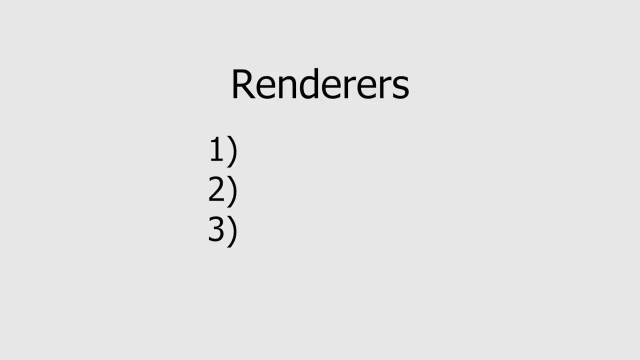 A renderer simply takes a 3D scene, which might have triangles, spheres, lines, etc. and renders them to a 2D screen, since unfortunately, we don't have holographic displays yet. There's three types of renderers I'll talk about today. The first is by far the most.